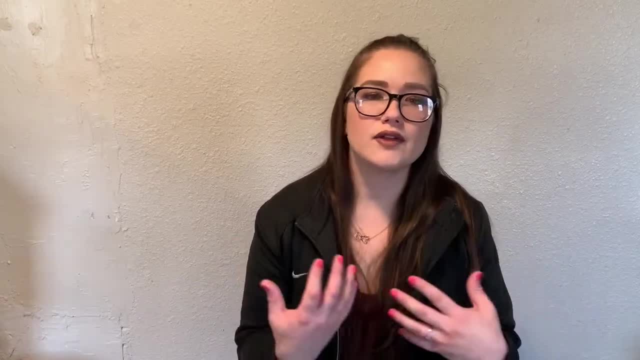 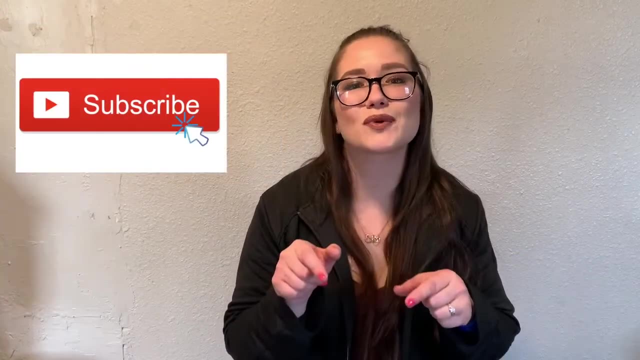 I'm going to do a little bit of math. I'm going to do a little bit of math. I'm going to do a start this series where I'm bringing you everything that you're going to need to teach math remotely. So if you're new here, go ahead and hit the subscribe button and the bell so that you 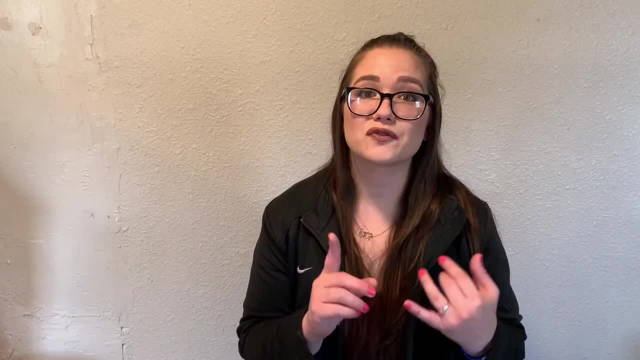 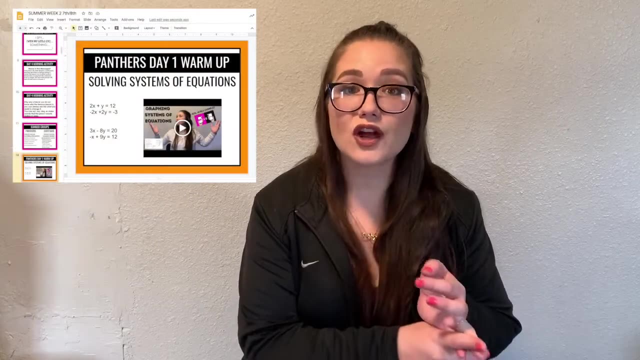 are notified and you won't miss a future video. I make videos for students, parents and teachers interested in sharpening or extending your math skills. If you're a teacher that wants to use technology or embed videos into your lessons, or if you're a parent who just needs resources. 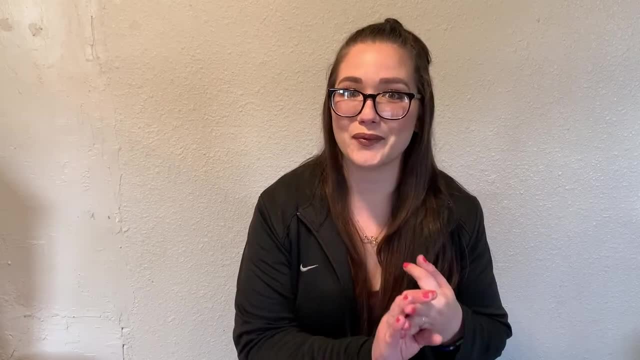 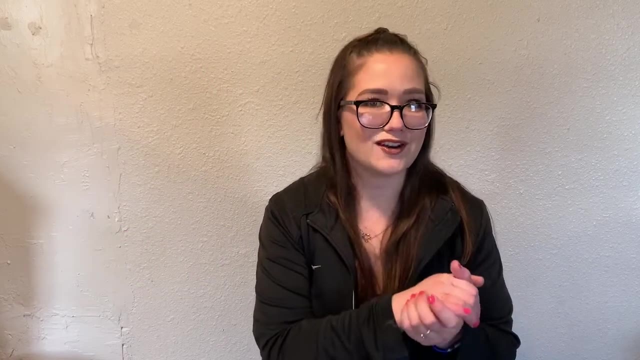 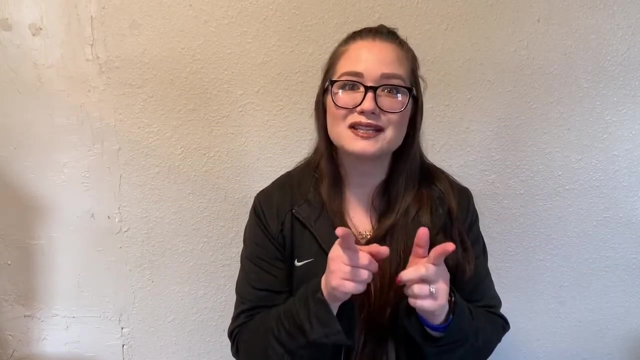 or refresher lessons do help your child at home. So that is why I made this channel: to help parents, teachers and students with math-related content. If you guys are excited, just like I am, go ahead and hit the like button and let's go on and jump into how to teach math remotely in 2020.. So, first things, 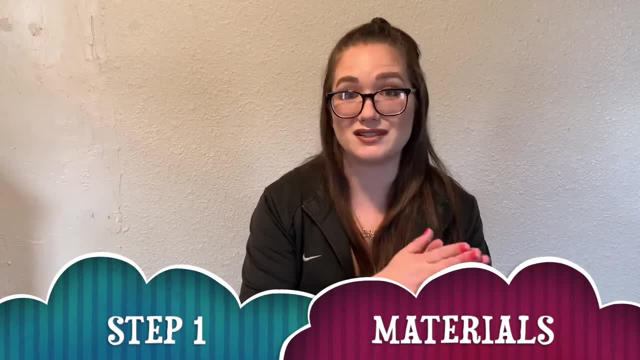 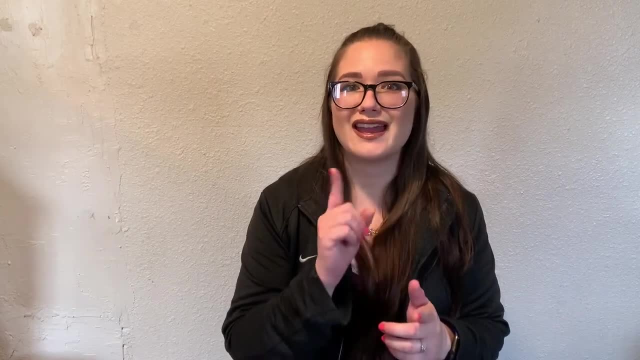 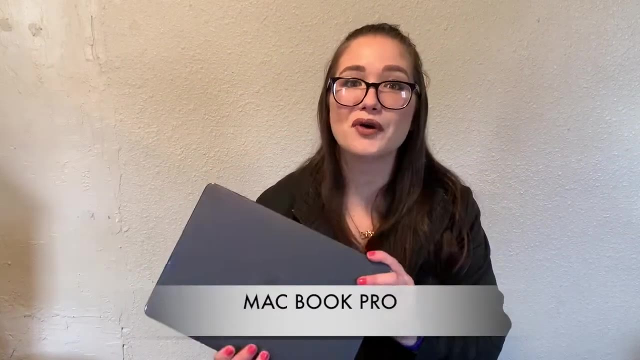 first we're going to talk about what materials that are going to help you be successful at teaching a math lesson to your students. So the first thing that I use is a laptop. So the laptop that I use is just the one that my school has provided. It is a MacBook Pro. 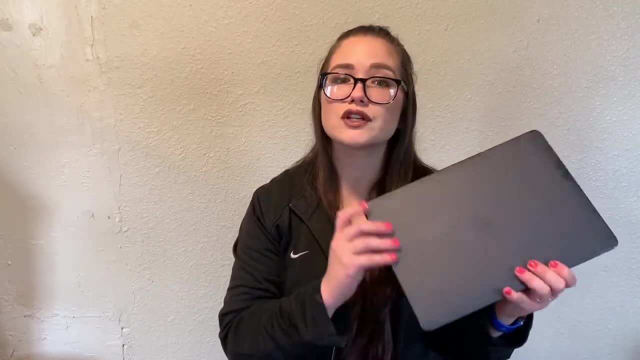 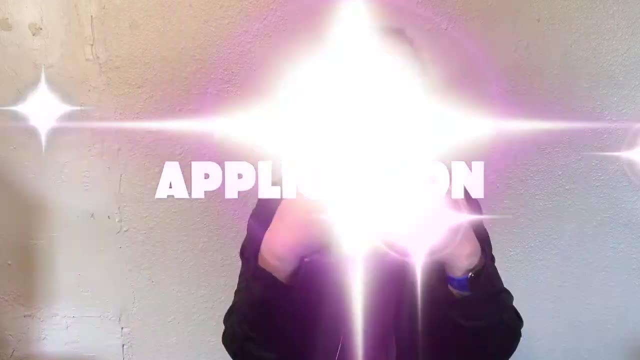 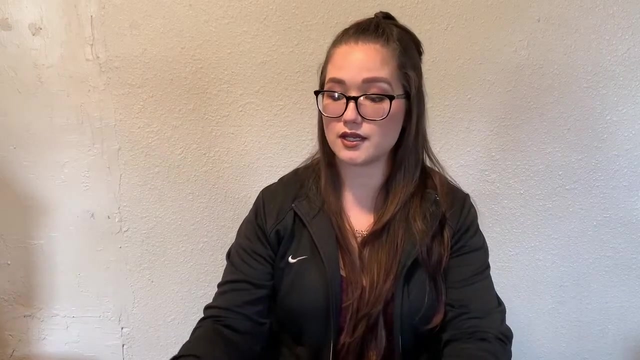 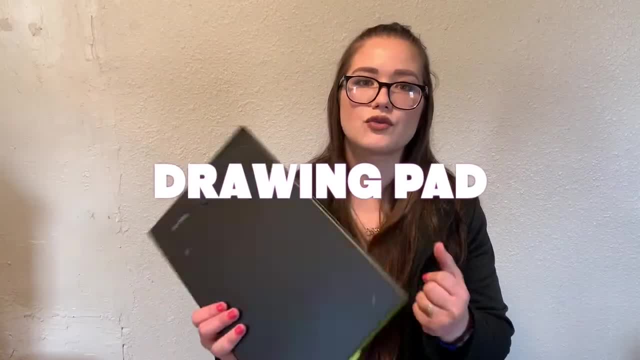 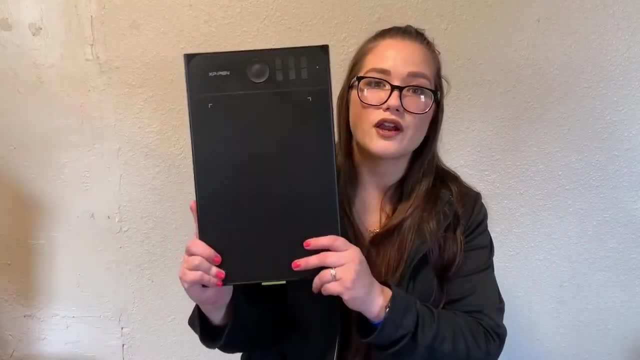 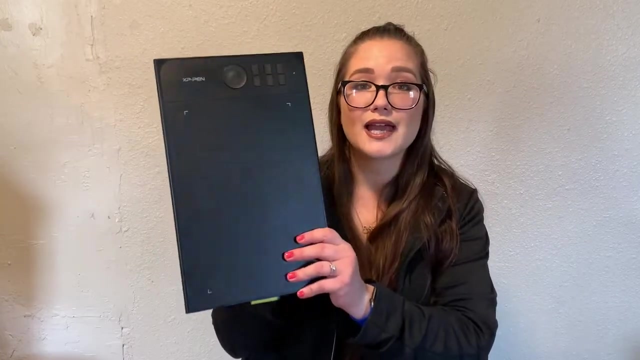 hopefully use this during this lesson. However, what my math lessons are so successful is a drawing pad, So this is the drawing pad that I have. I know there are a lot of different brands out there. Sorry, excuse me, it's a little dirty, But this one is from XP-Pen. I will link one down below. I got 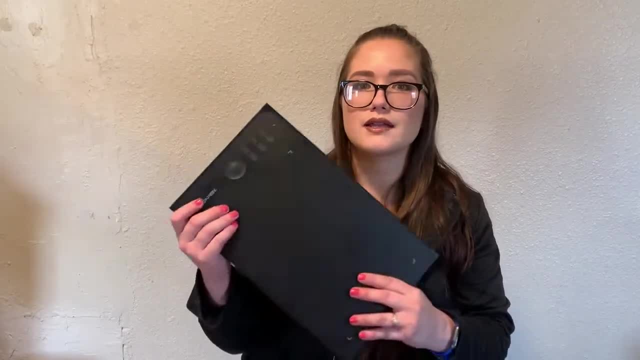 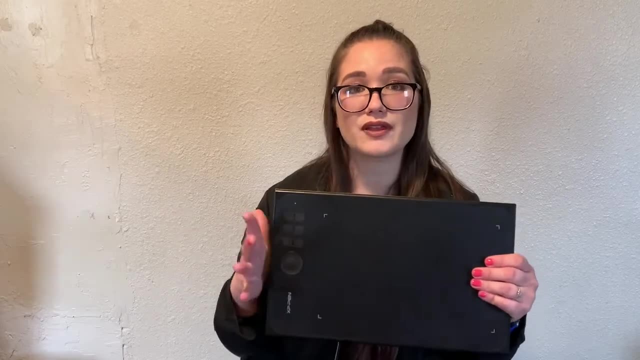 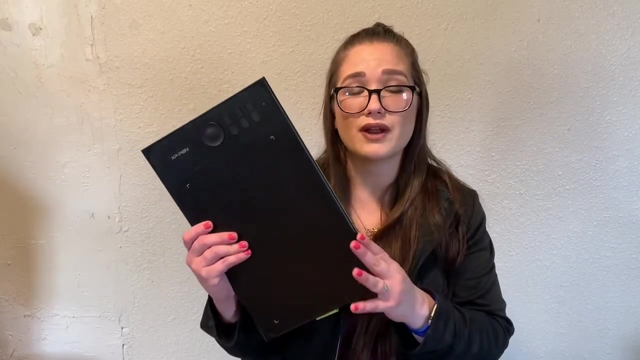 it off of Amazon. But this is amazing, It has buttons on the side, little shortcut buttons. I do not use the buttons on the side just because of the app that I'm going to talk about next, but yeah, this was a really good investment. XP pen is a really good brand and it's it's a lot cheaper. 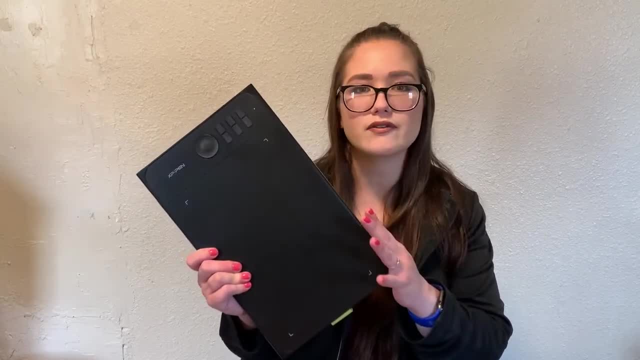 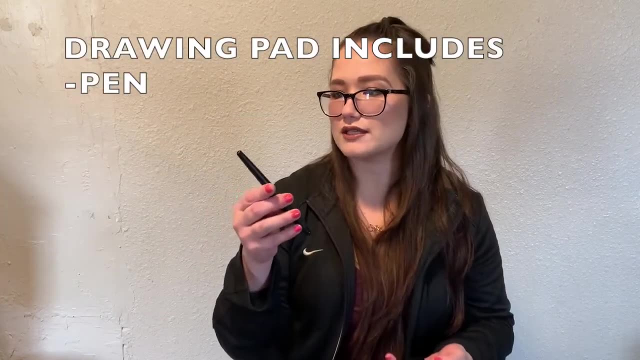 than the other brands that I've seen recommended and it hasn't given me any trouble. I have nothing but good things to say about this and with the drawing pad it came with this pen. um, the pen comes with a little stand, so when you're not using it, you can either stand it up like that. 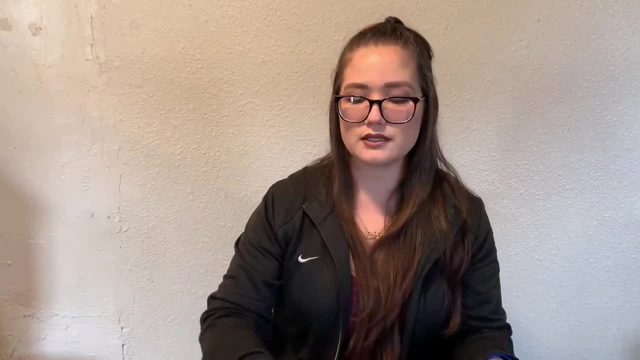 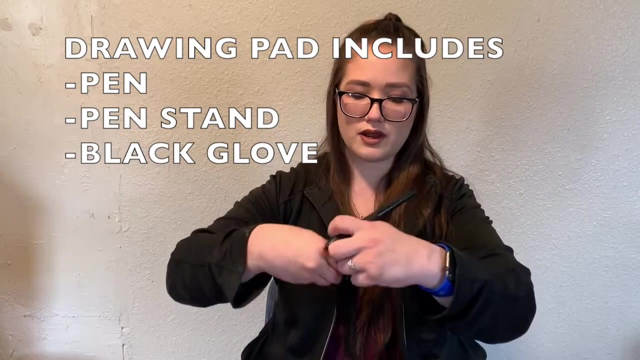 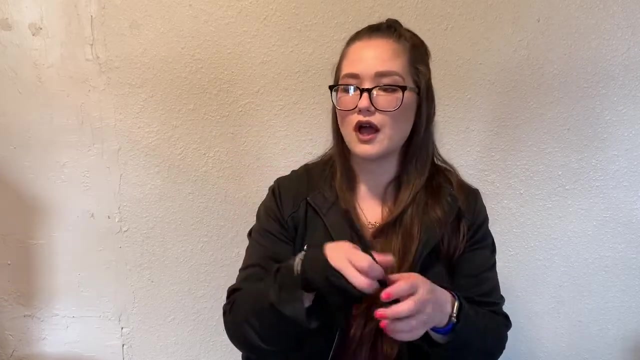 or lay it down this way. it also comes with because it's a surface where it's very touchy. it comes with this um glove that you can wear. it has two fingers so that when you're writing your skin is not touching the pad. so it's, and it's, very comfortable. um, it also came with a little. 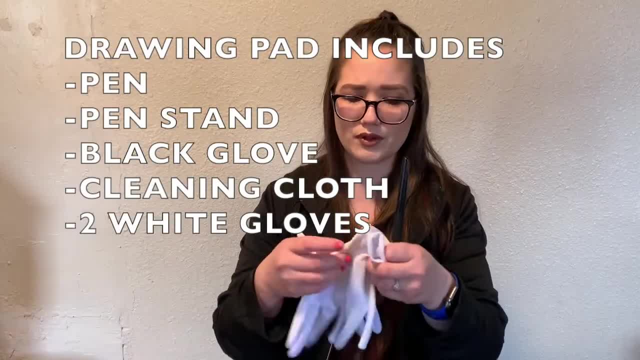 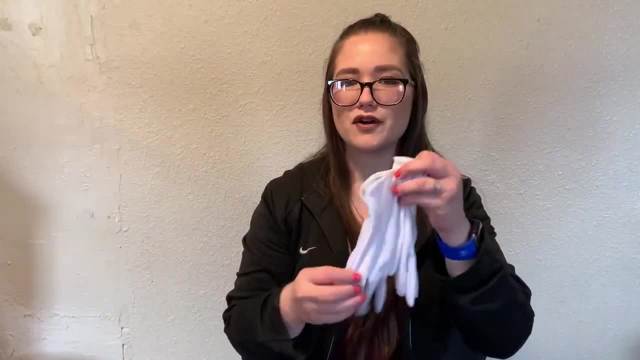 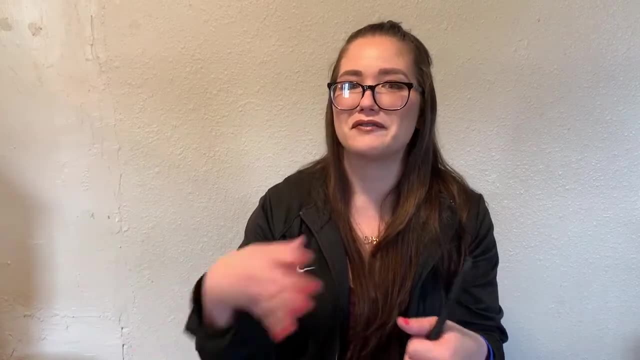 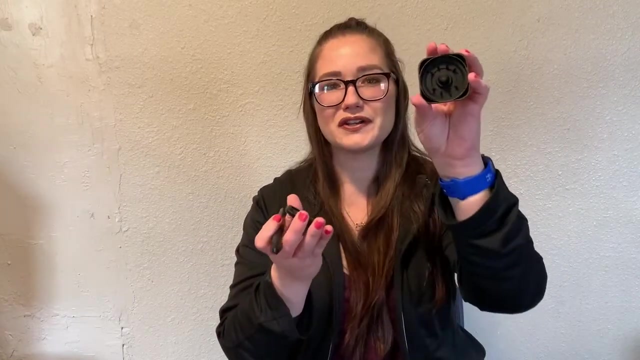 cleaning cloth. um, and it came with a couple of white gloves that have these, um, like textured dots on them. it's kind of rough on one side and very smooth on the other. not exactly sure what these are used for. I don't use them, um, however, it came with the kit, so that is what I'm showing you. um, so there's also little. 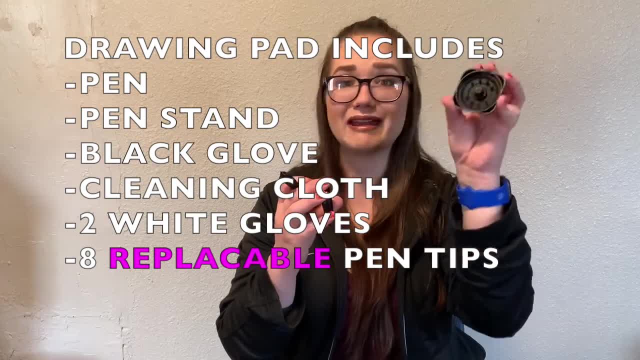 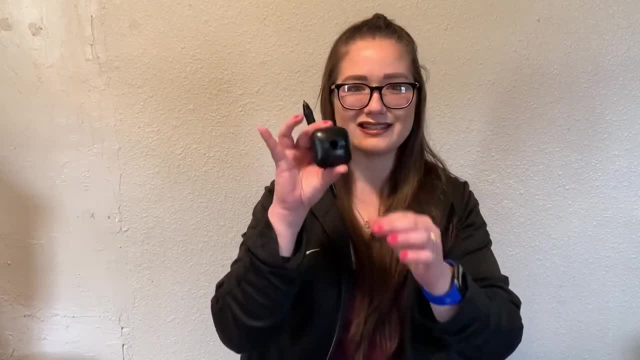 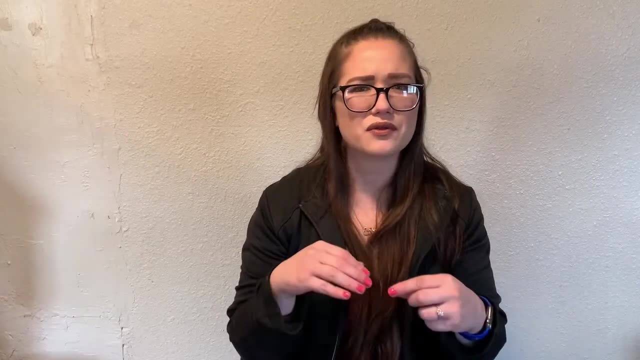 tips. on the inside there's like six, eight, um refillable tips. I guess you can call them um in the um pen stand. so I thought that was pretty cool, uh, that it came with that. so I think the price for this I don't, I don't want, I want to say I didn't pay more than forty. 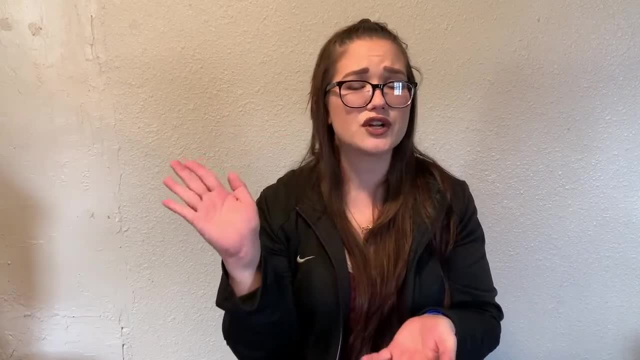 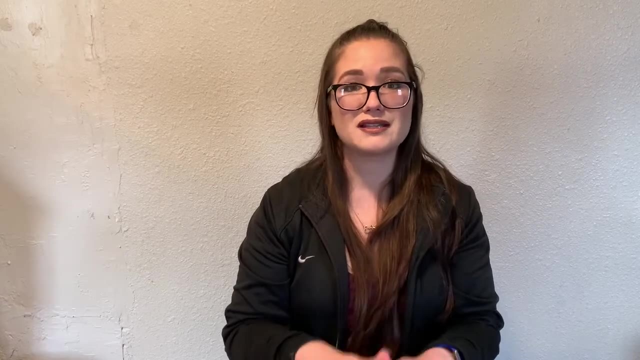 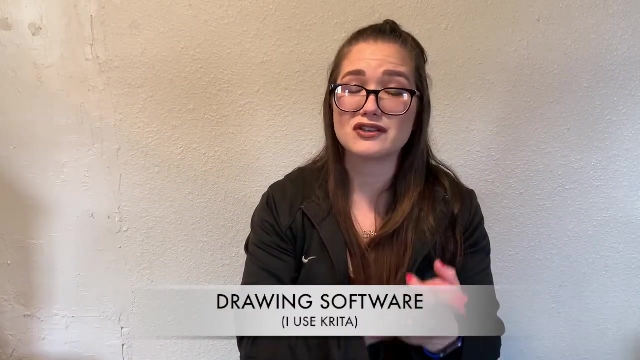 dollars for this. I know there's some that range over a hundred and there are a few that are less than 40.. like I said, this one is really good. I definitely recommend it. um, the next thing: you are going to need a drawing software. I spent a lot of time researching the different drawing softwares. 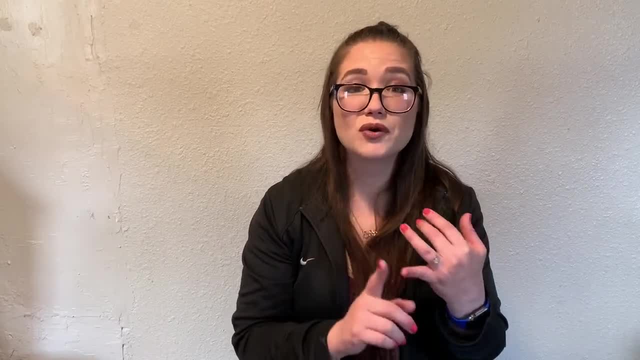 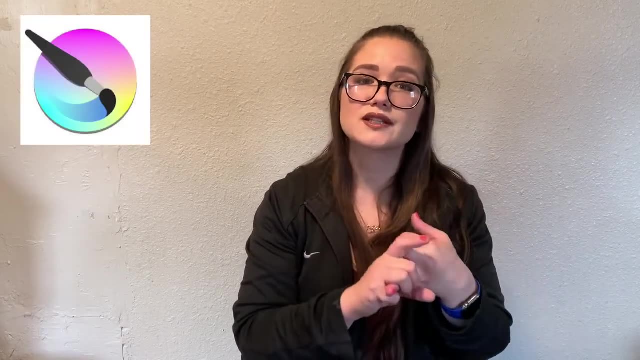 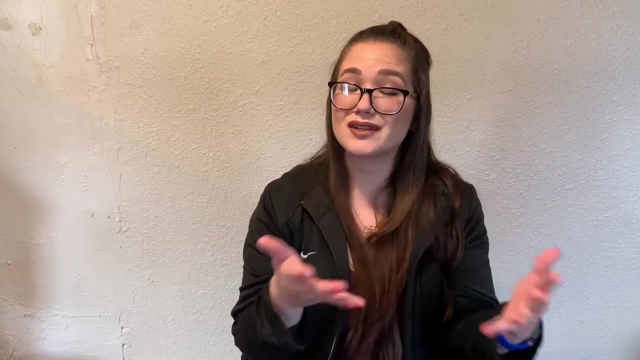 the one that I found that is the most user friendly but the most features. I like using Krita um. Krita is a drawing software that you can use for iOS and PC, so it works for both. it's just really easy. I'm gonna um throw a clip in right now where you can see. 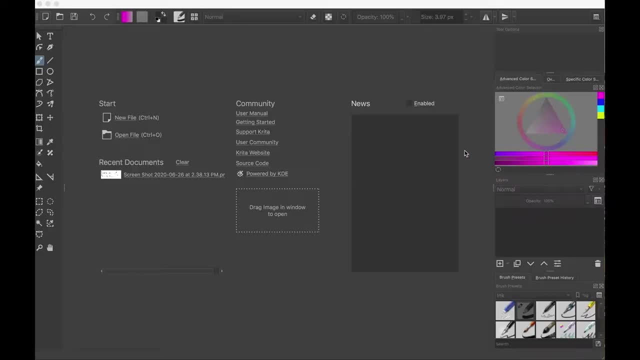 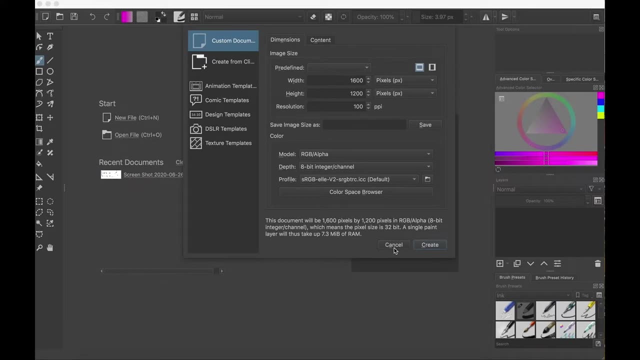 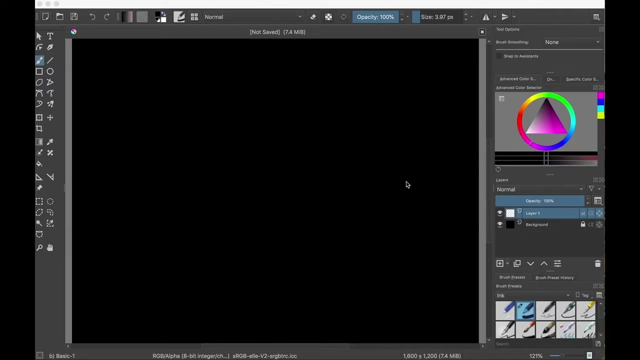 it in use all right. so I just wanted to show you really quick. this is what it looks like when you open Krita. um you can easily just start a new file this way and create a custom document. um, I set up my settings so that my screen comes in black. I just um the students like: 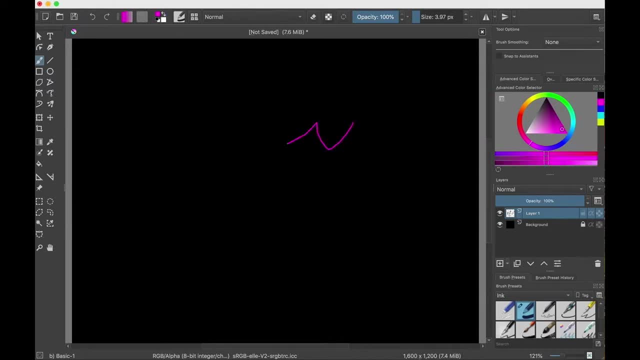 um the writing on it, better, just the brightness of it. um. so the colors are over here. they're, um, just the colors that I use frequently, so I can quickly change back to the colors that I always use. if I wanted to open a new screen, I just come to the new button. 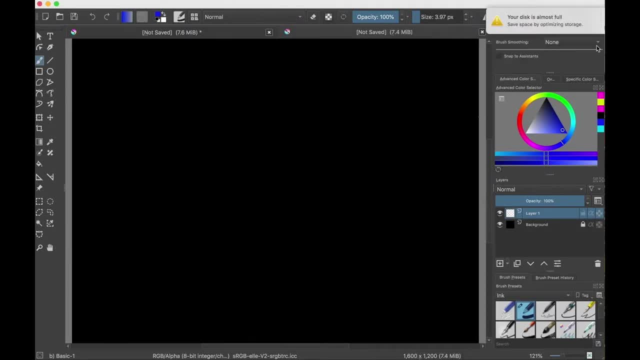 I click create and, um, sorry, my, my memory's almost full um, but yes, I come to the new button up here. I click create new and you can do as many of these as you want and you can come back up here. let's say, I saved an equation that I wanted um on that one. and then I come over here and we do a little. 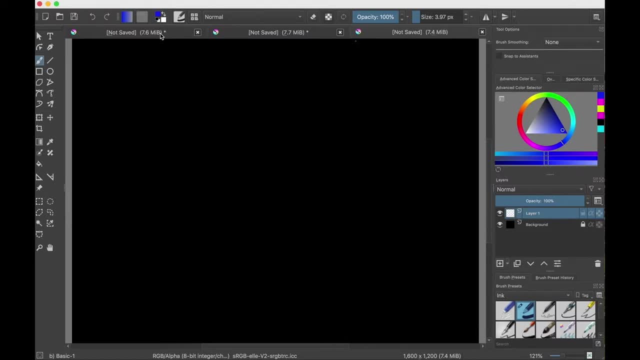 drawing or not drawing. but another equation: um and I come over here and I have something else saved up here that I want to go back to. um, what's also cool in this is, if I wanted to get a picture, this picture I just took from our online curriculum we use. 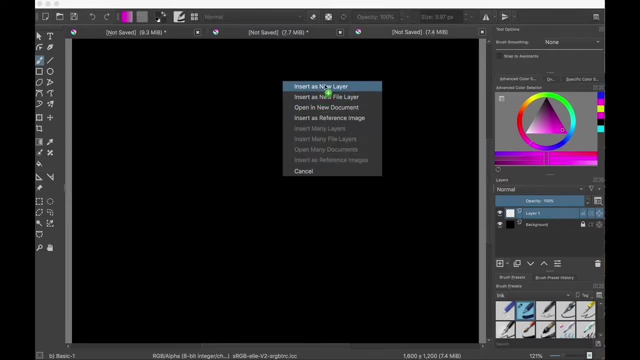 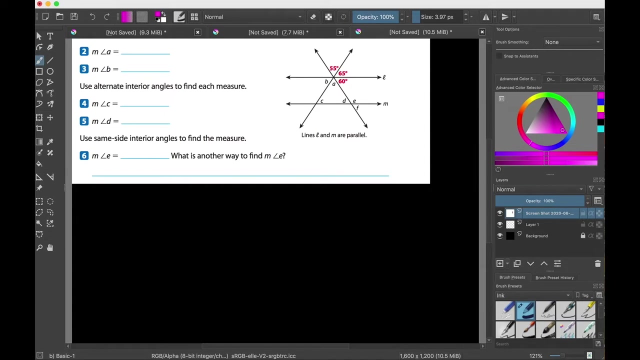 I ready at our school, so I screenshot a picture and I can insert it as a new layer. I can insert it as a file, a new file layer. um, either way you do it, if I insert it as a new layer, I can draw right over it. if I'm talking about angles, I can draw on it and show them the vertical. 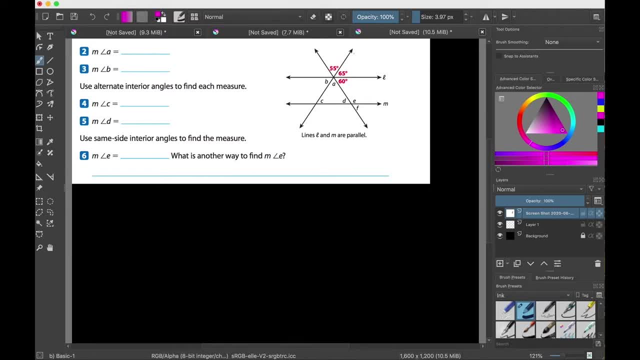 angle. and again, this is good for virtual learning because you can actually- the kids can actually see the textbook with you, you can draw on it just as you would if you were up in front of the classroom doing it on your document camera. so I really like that. and then also you can use the space. 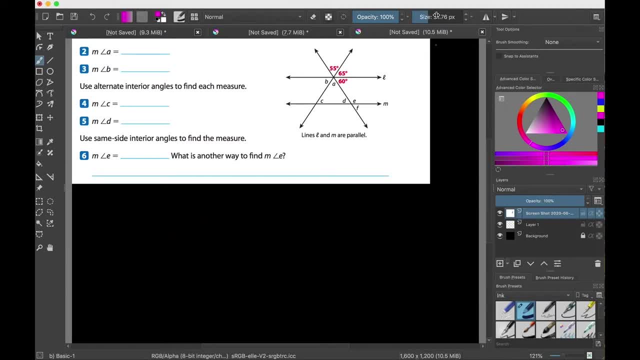 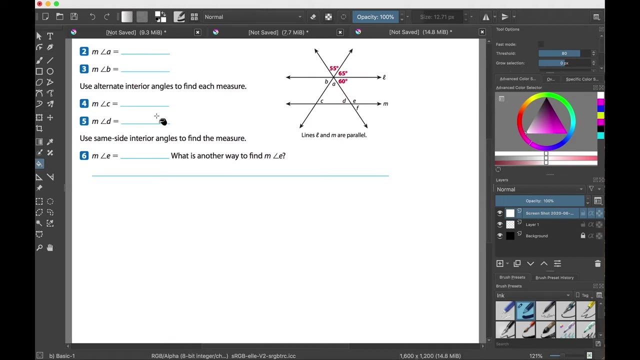 down here for extra drawing. you can change the size of your pen down here. you can change the type of pen you want. you can draw shapes and, um, yeah, there's nothing uh limits you in this program, so you can make it a white background. like I said, I like black, um, just. 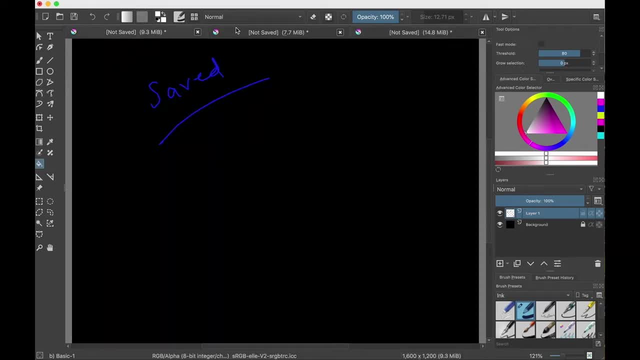 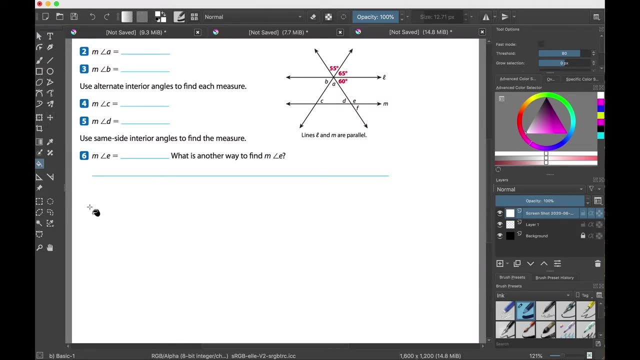 because my students said they preferred it. um, but yeah, I mean, there are a ton of things that you can do. I record from here and I put it up on my Google classroom. um, and the students who don't um have access or their internet is giving them trouble during the 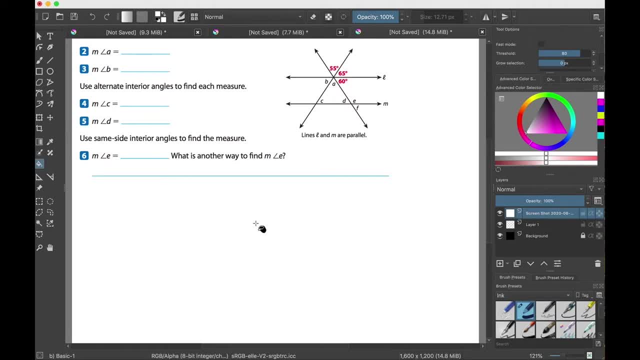 class time. whenever they do get a hot spot or they can get online, they can go on to the Google classroom and get the lessons virtually there. so I really like Krita for these reasons. check it out for yourself. it's totally free. it works for iOS and and Windows, so check it out, I love. 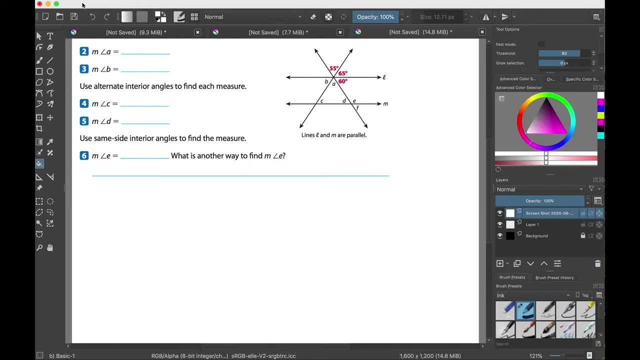 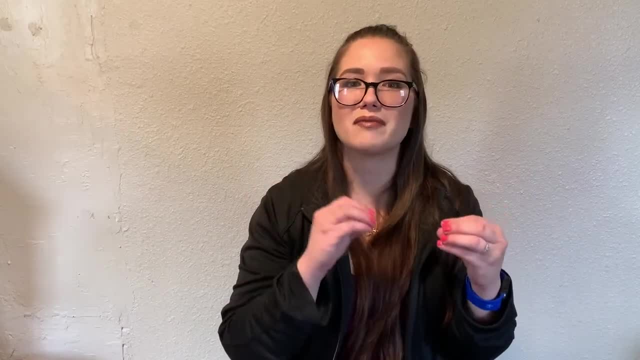 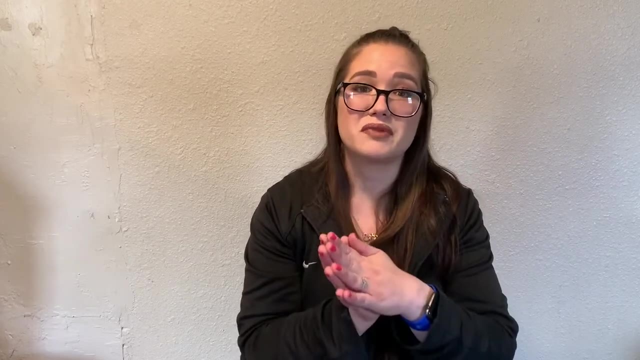 it. look uh for the link in the description down below for the drawing pattern and the iPad and the Krita website. they're both free and it's really made my math teaching and the students ability to um get support from me that much better, so I really recommend getting your. 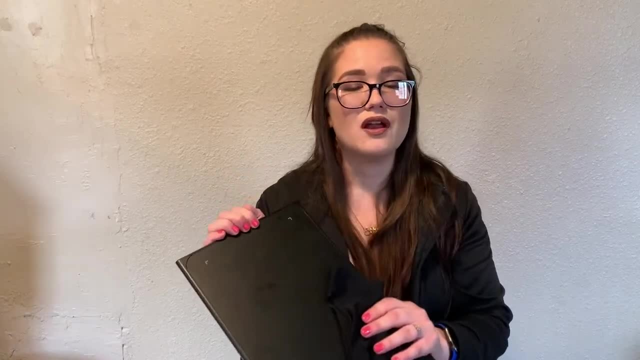 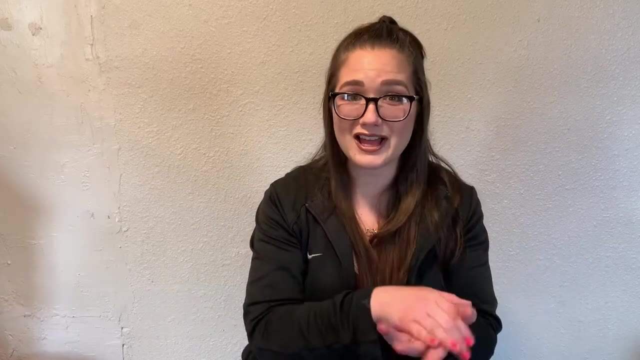 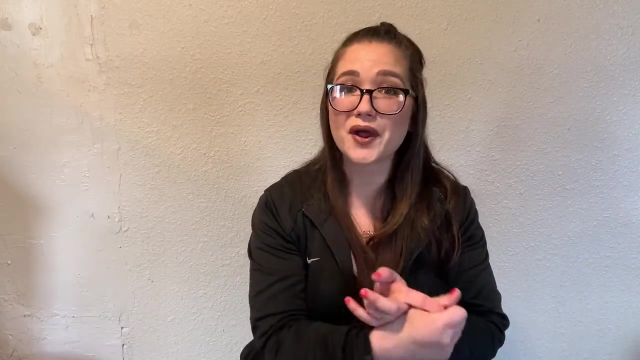 drawing pad and your drawing software. um, with that being said, the next material is going to be your lesson plan, or your notes. to teach math online effectively, you're going to need to be prepared, um, so coming with your lesson already done is going to be a priority. make sure you have. 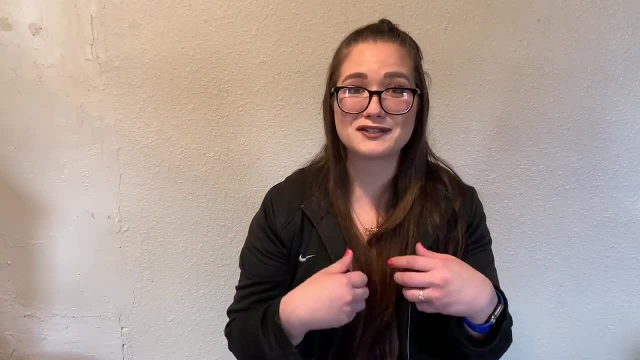 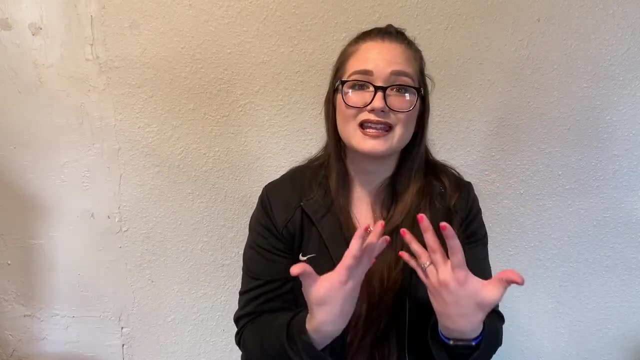 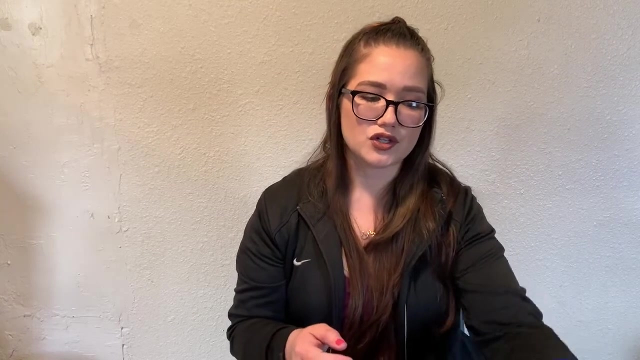 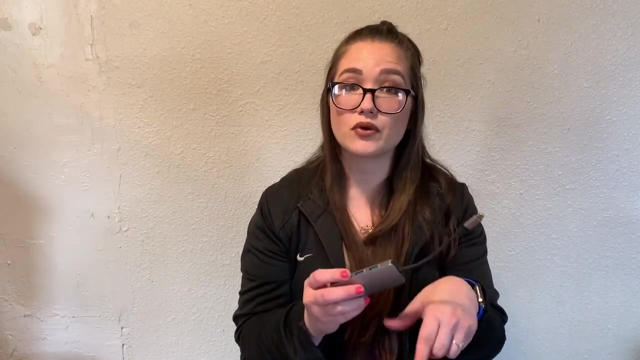 everything ready, um, so that when your students log into Zoom you're not scrambling getting everything ready, you're prepared, and it makes your students feel more relaxed and at ease knowing that you have prepared this thought out lesson for them. okay, uh, the last thing I want to show you is the C cable, um, so I did need an adapter because my drawing 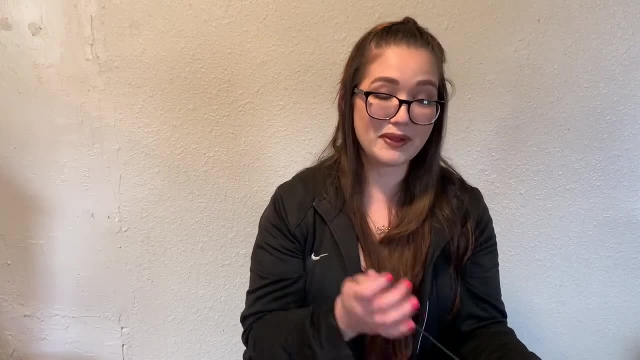 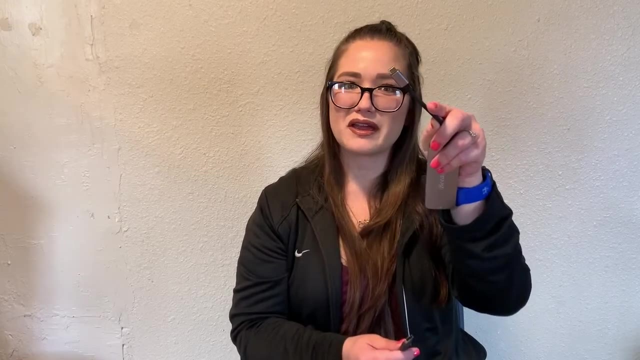 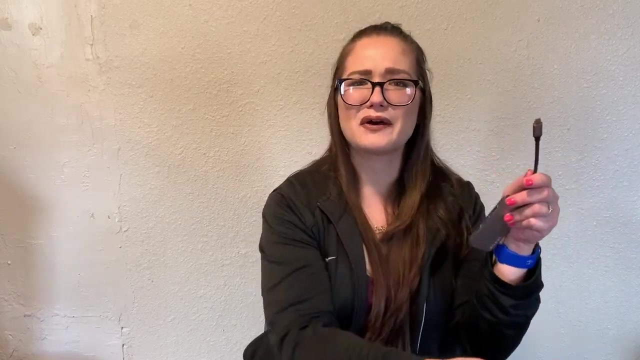 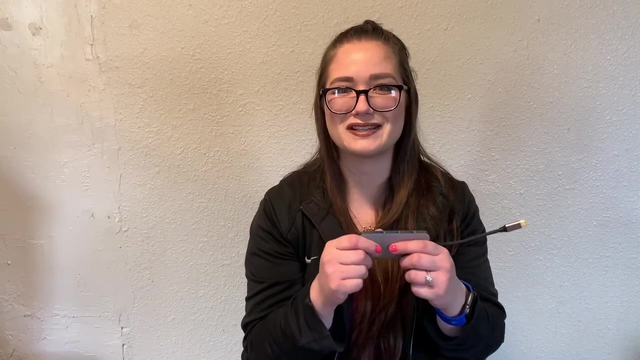 board, the x-pen drawing board. it has a USB plug at the end of it, so I needed to buy a USB adapter that would plug into the C end of my computer and the um. the USB adapter can go into that. so I am not very technology savvy when it comes to um what the names of the cords are, so excuse. 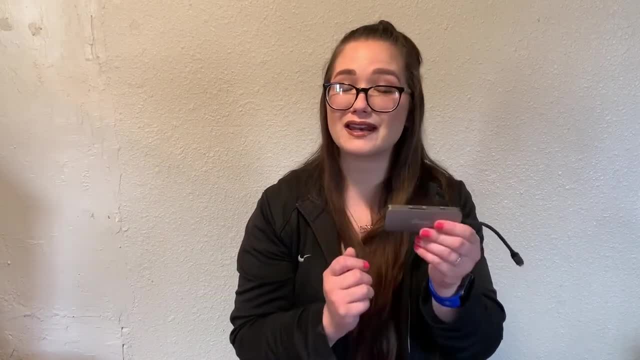 me if I said that wrong, but, um, you might need an adapter depending on what you're using, and we're going to go ahead and get started, but I think you can do that here and, yeah, I would recommend you try to use this if you want to use it. 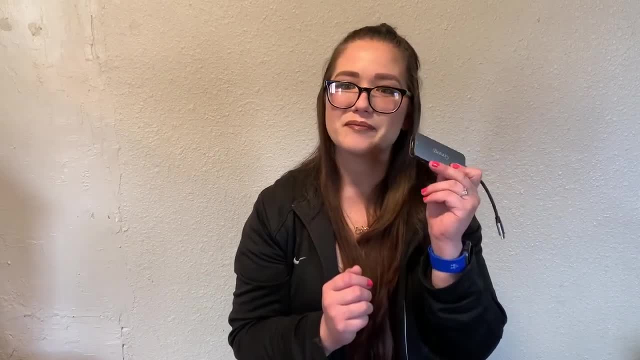 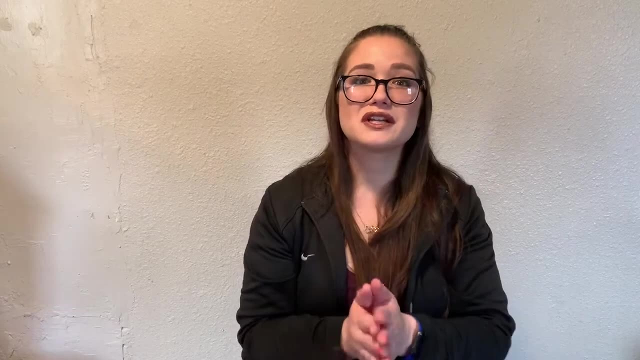 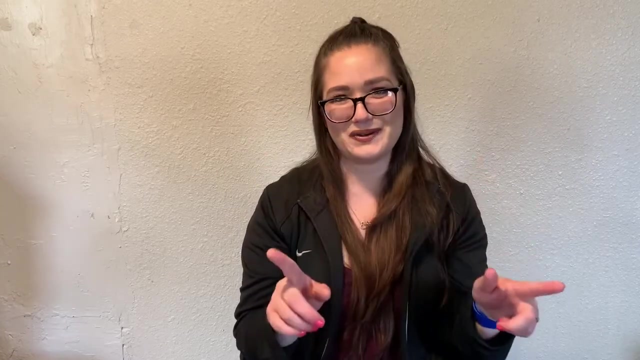 your laptop or whatever device you're using, um is capable of using, so just keep that in mind. all right, so that does it for materials. the next thing that we're going to jump into is the steps to teaching math effectively online in 2020. okay, so, let's get into those steps. all right, so teaching. 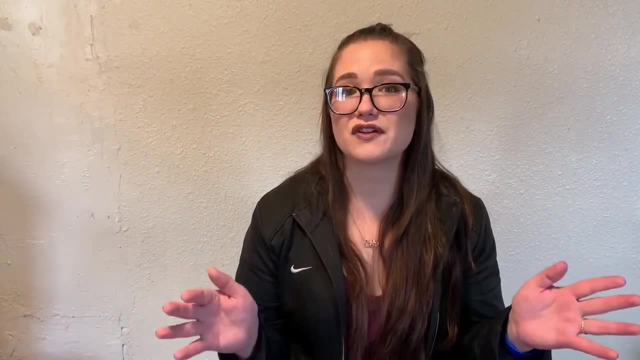 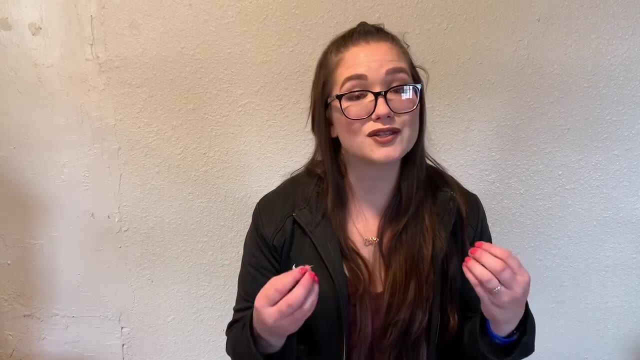 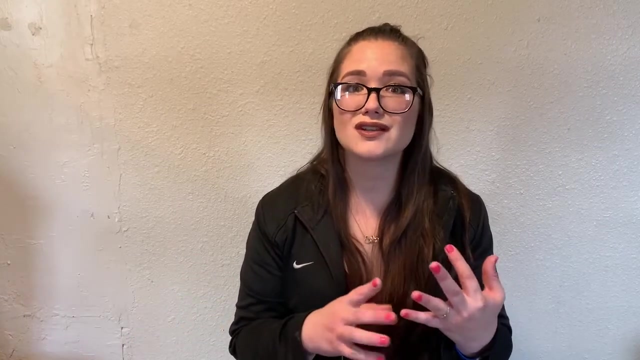 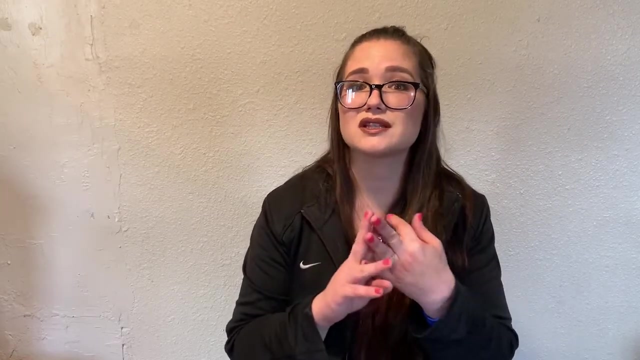 math effectively online. it can look very different for one person um to the other. it just depends on what materials you have available to you, as well as what your students have available have available to them. some students don't have internet. some students internet doesn't work very well because um the other family members are using the internet at that time. some students are. 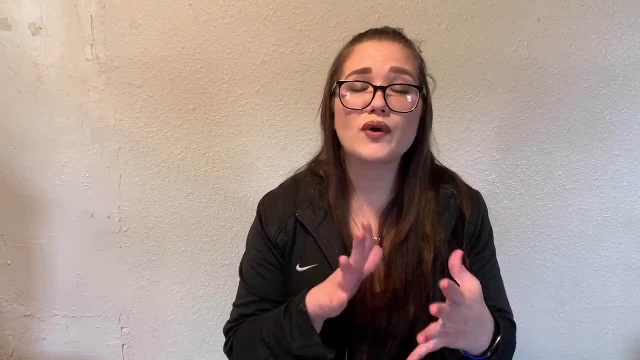 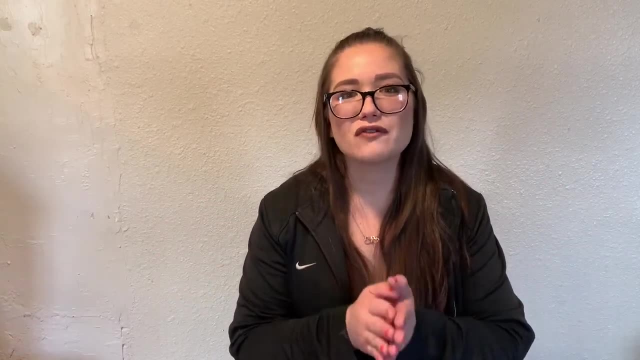 trying to log on and then their internet crashes. so there's always something, and you need to be prepared for all of it being a teacher. so i want to go over some steps for you and i'm going to give you some tips and tricks to help you get started. so let's get started. so let's get started. 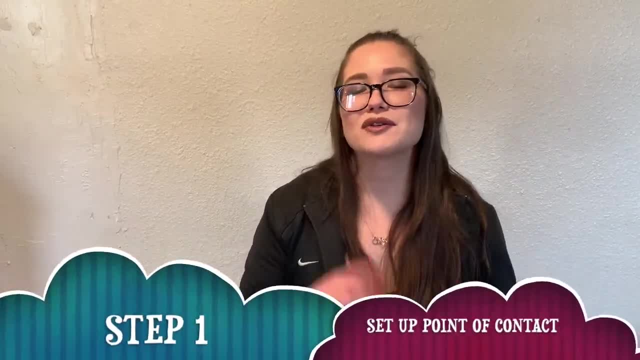 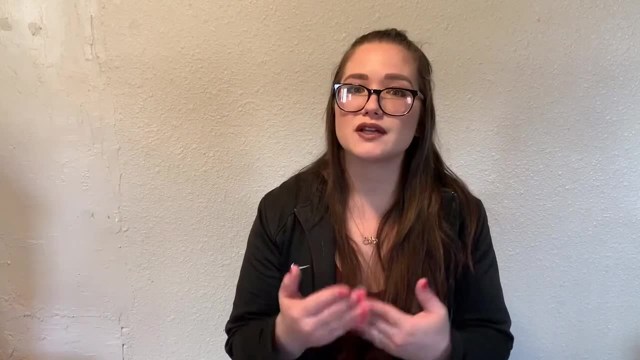 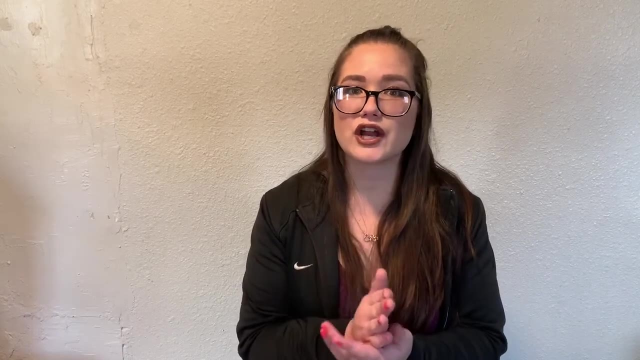 some different variations in case things like that do happen. so step number one is to set up that point of contact. so, whether you're using zoom or whatever app that you're using, i'm just going to go from what i have experience with. so, um, having the links ready, shared out with. however, 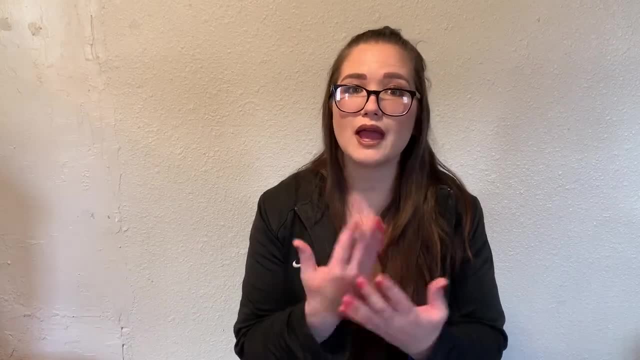 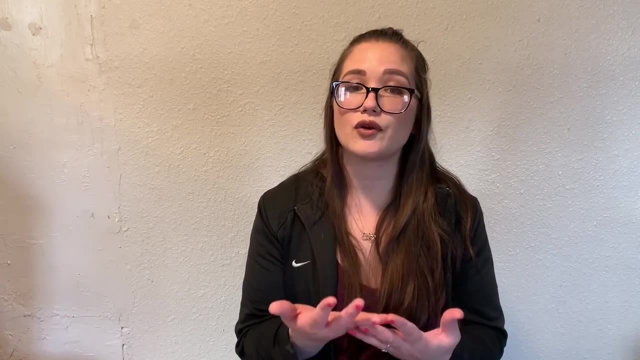 you communicate that with your students. i have a google classroom and i share out my links to the zoom meeting at least a day before so the students know and are prepared and are ready to go to the zoom meeting at least a day before. so the students know and are prepared and are ready to. 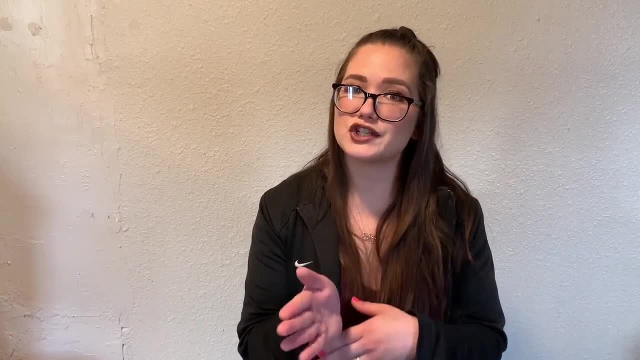 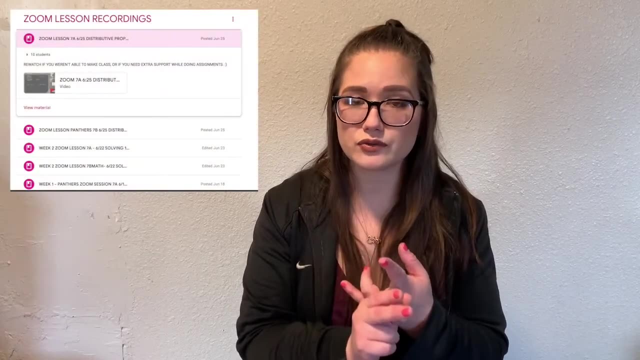 go to the zoom meeting at least a day before so the students know and are ready to go if you are not meeting live. so this is your variation: you can record yourself doing the lesson, um, you can upload that video of you doing the lesson to your google classroom or whatever. again, whatever app that you're using, but you can. 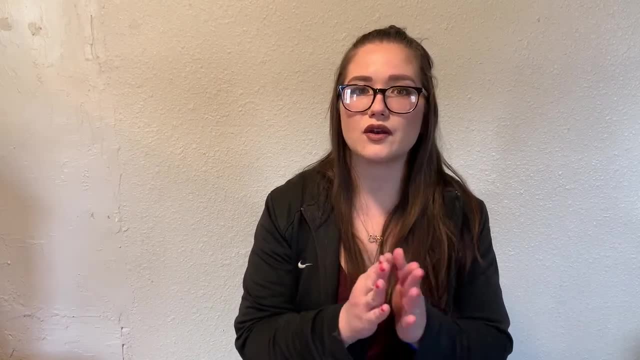 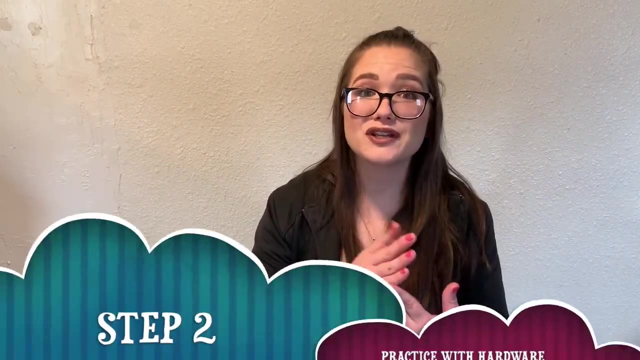 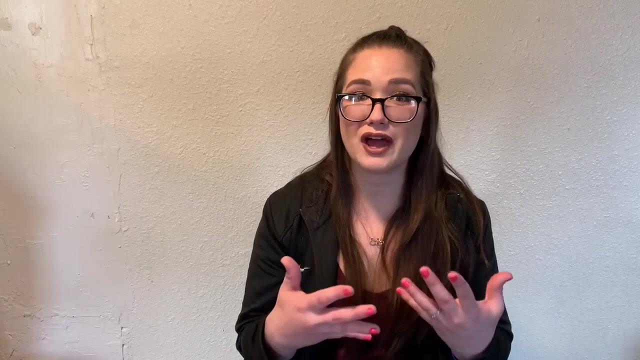 upload you doing the video so the students can watch your lesson and take notes so that they're able to do the work that you're assigning. so step number two is to practice with your hardware. so, um, so the worst thing you can do is get in front of your students and not know how to use the. 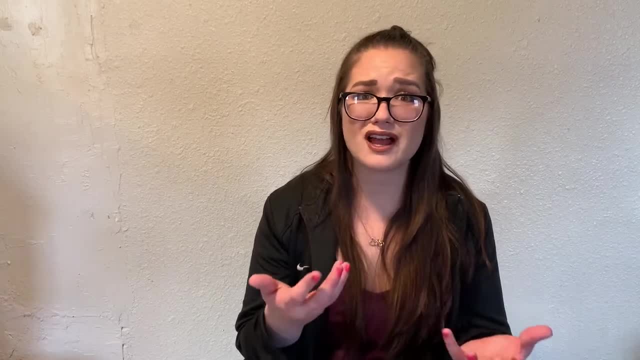 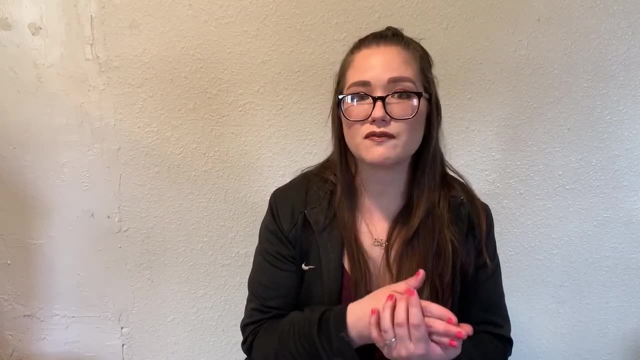 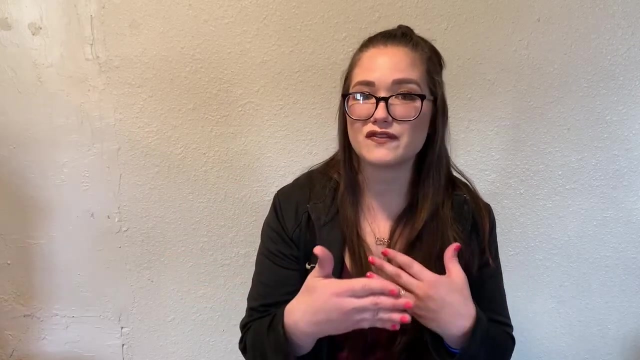 software or the hardware that you're using, um, and you take 20 minutes of class trying to fumble around and it's just um not as professional as to take a few minutes before you get in front of them to learn all of your materials. you never know who else is listening behind the camera when. 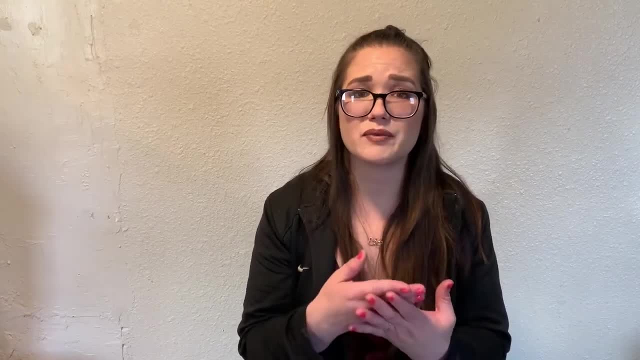 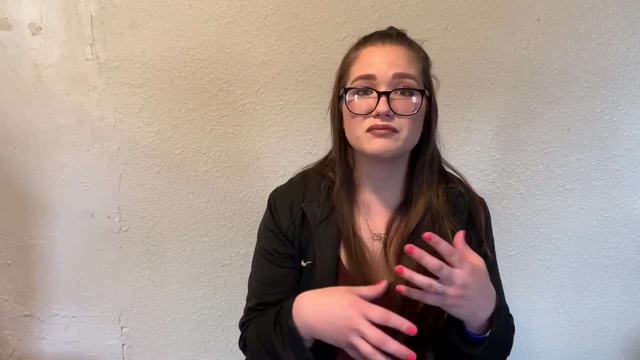 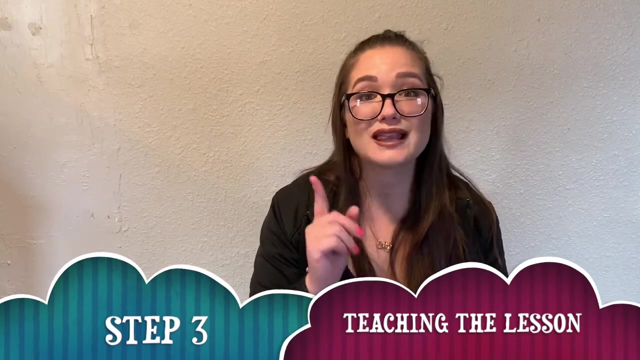 you're teaching face to face online, so you always want to make sure that you're prepared. practice run, ask somebody in your family, create a zoom link and um, work out all of the kinks first before you get in front of your students. okay, so step number three is the actual lesson. 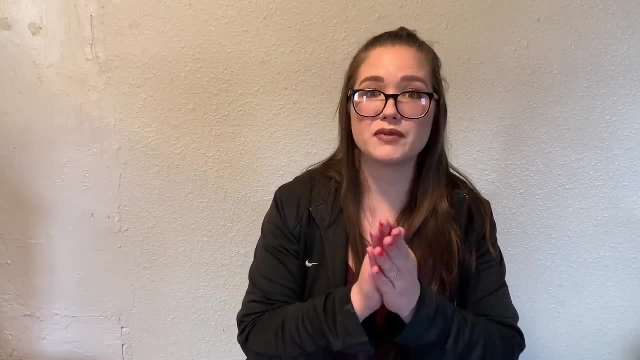 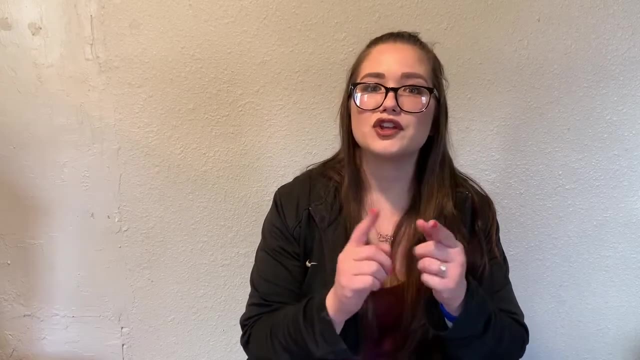 so teaching the lesson online. um make sure, before you get in front of your students, make sure you set up the settings that you want in your zoom during the actual lesson. um utilize things like the chat so make sure they're being engaged. say things like hey, if you're, if you're with me, type. 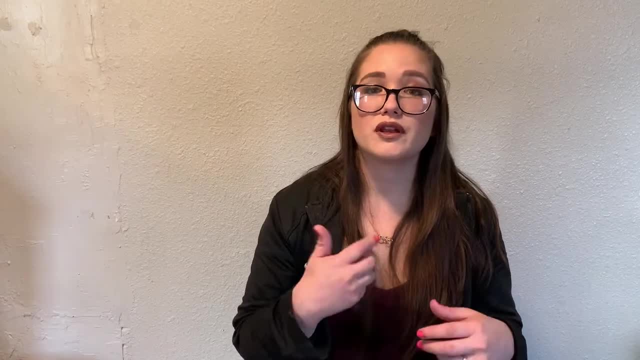 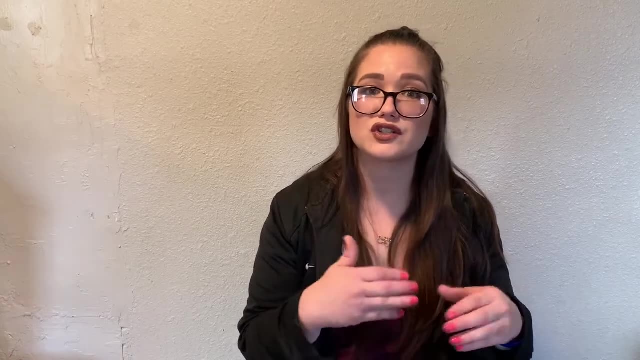 a yes in the chat and make sure everybody is with you. you can, if you have an assistant that's in your zoom, you can make them the host for a little while and type little messages to each student to make sure that they're checking for understanding while you're doing the lesson. 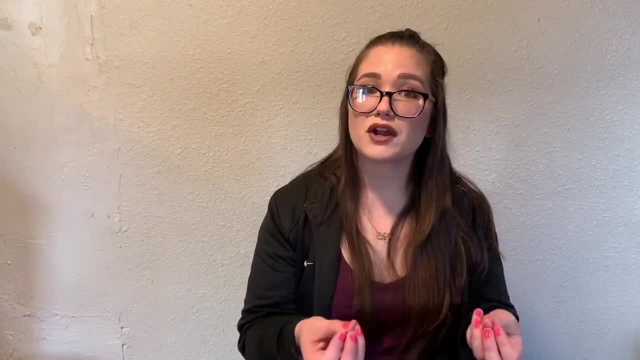 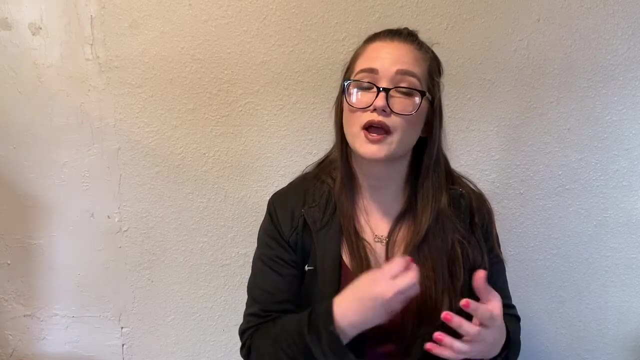 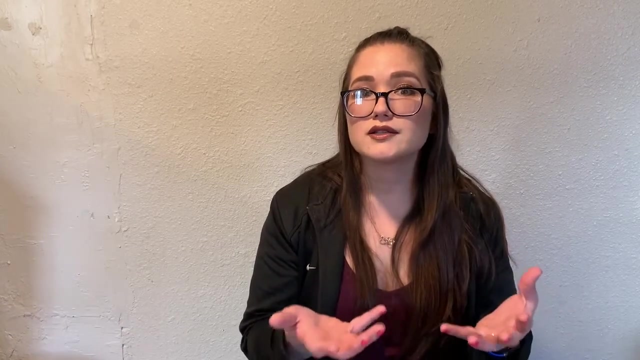 also keep in mind that some students don't like to share through their microphone. they would rather type their answer versus say their answers. so you know your students more than anybody, so make sure, if you have students like that, to allow them to feel comfortable typing their answers instead of verbally saying their answers. um, so yeah, just keep all of those things. 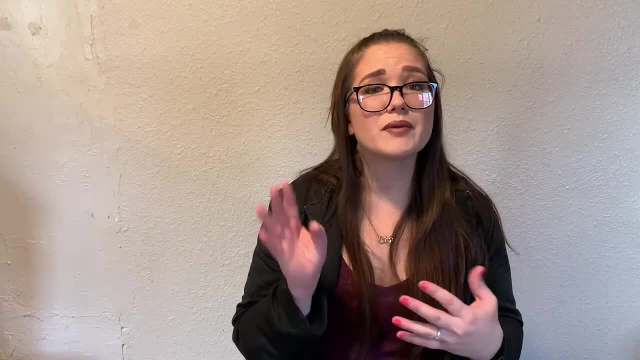 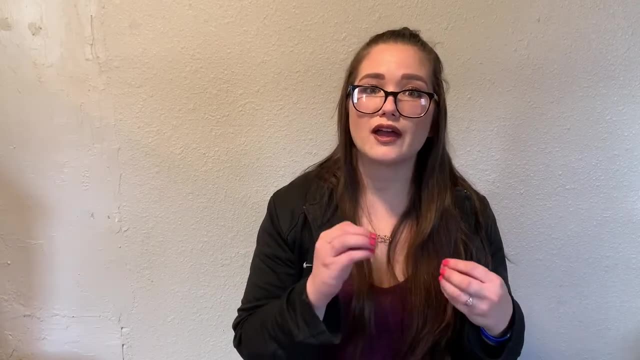 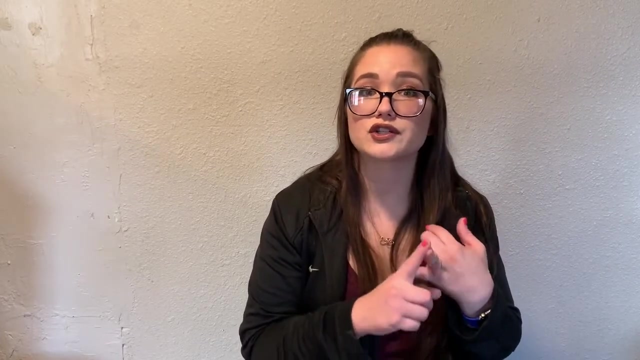 in mind for during the lesson. okay, so, and then step number four is to provide feedback. so, as your lesson is going on, making sure that if they're answering the questions, if you're having them turn in work or turn in their questions online, maybe it looks like them turning their 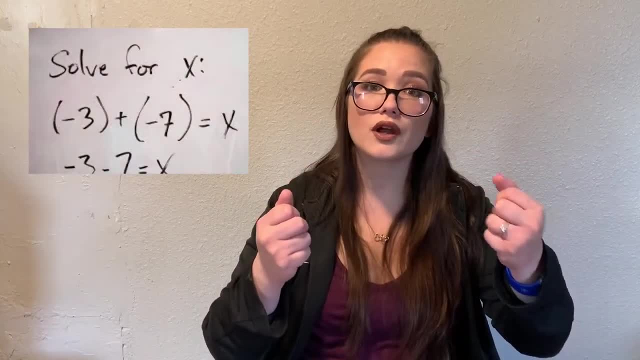 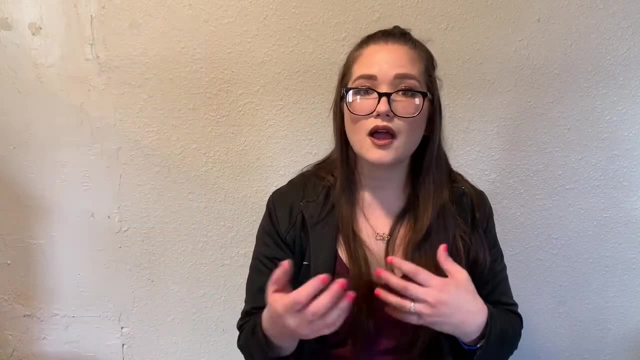 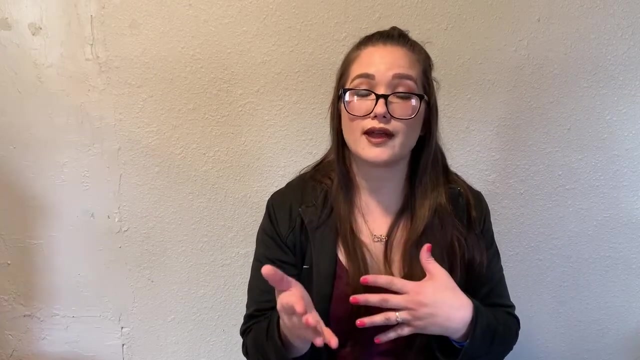 cameras down or picking up their books and just showing you their work. maybe it looks like them taking a picture of their work and submitting it to an assignment on google classroom to be graded- however that looks like, but provide immediate feedback. i like to record the lessons on zoom and then put the recordings online so that if